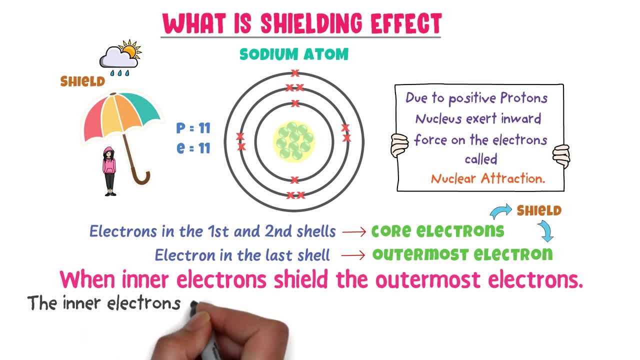 Also, we can define shielding effect as the inner electrons shield the outermost electrons from the nuclear force and reduce the nuclear hold on them. This effect is called shielding effect or screening effect. Secondly, we can also define shielding effect on the basis of Coulomb's law. 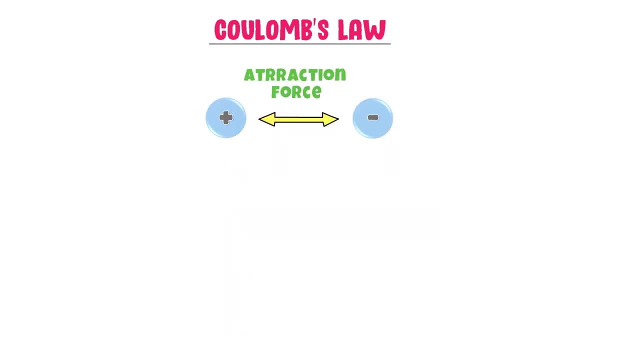 Coulomb-Baba states that there is attraction force between proton and electron because these both are charged particles. Let the distance between them is r1.. Consider another: proton and electron. There is also attraction force between them. Let the distance between them is r2.. 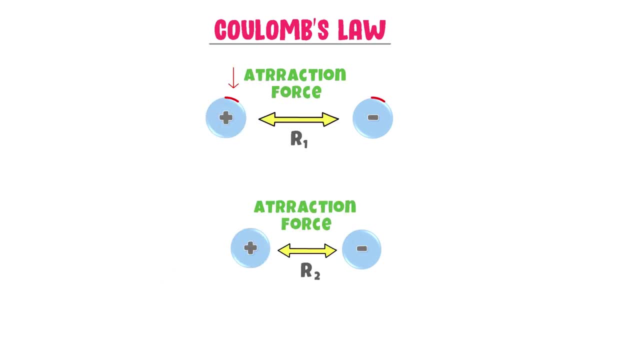 According to Coulomb-Baba, there is less attraction force between this proton and electron because the distance r1 is greater between them, while there is more attraction force between this proton and electron because the distance r2 is smaller between them. Therefore, in the light of Coulomb's law, we can say that outermost electron 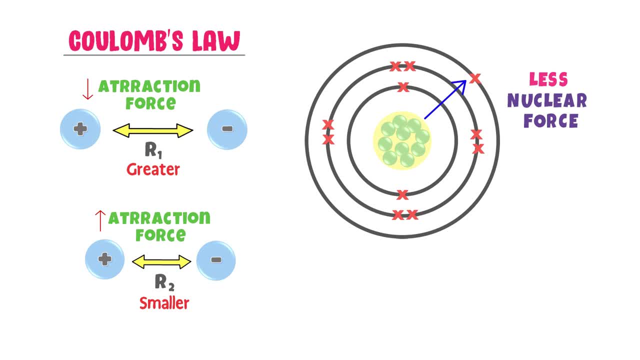 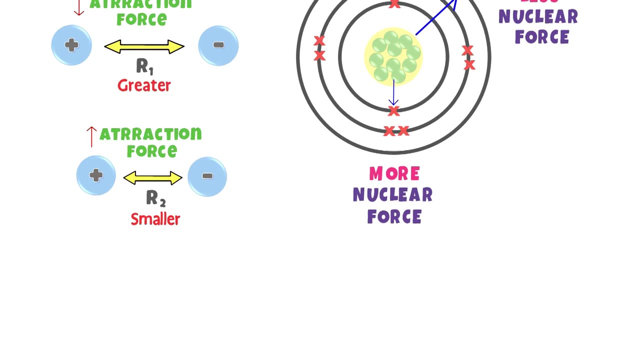 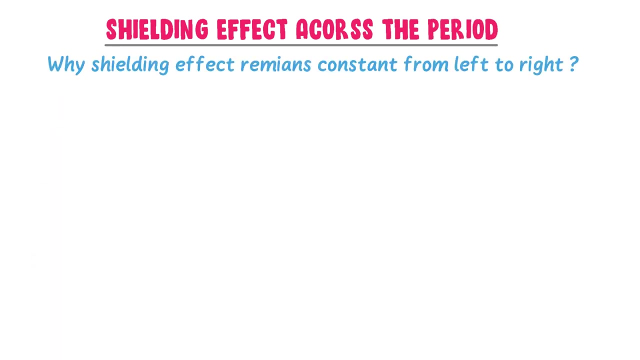 experiences less nuclear force because they are usually away from the nucleus, While the electrons in the first shell experiences highest nuclear force because they are near the nucleus. Now let me teach you trends of shielding effect in the periodic table, like shielding effect across the period, or why shielding effect remains constant from left to right in the period. 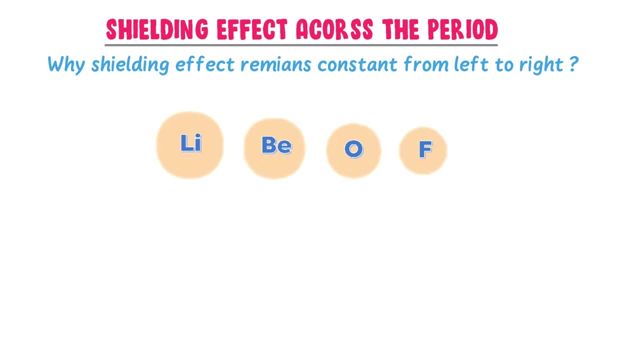 Well, consider the second period: elements like lithium, beryllium, oxygen and fluorine. There are two shells in the lithium, two shells in the beryllium, two shells in the oxygen and two shells in the fluorine. 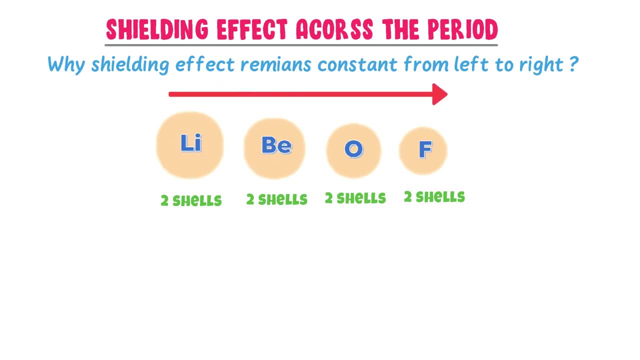 Thus the number of shells remain constant from left to right in the period. The valence electrons are round about at same distance from the nucleus. According to Coulomb-Baba, these outermost electrons experiences almost same nuclear force. Although the atomic number increases, it does not mean that they are almost the same. 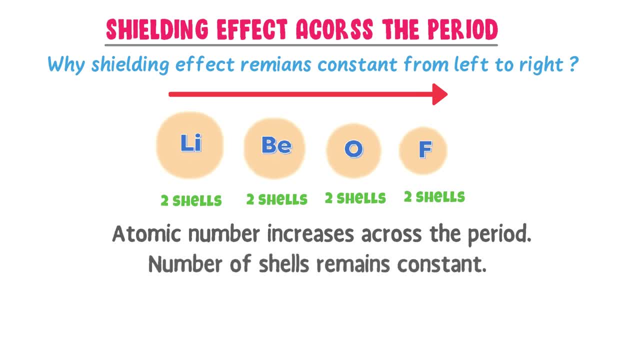 Although the atomic number increases, it does not mean that they are almost the same. Although the atomic number increases, it does not mean that they are almost the same. However, the number of shells remains constant across the period. But the number of shells remains constant.